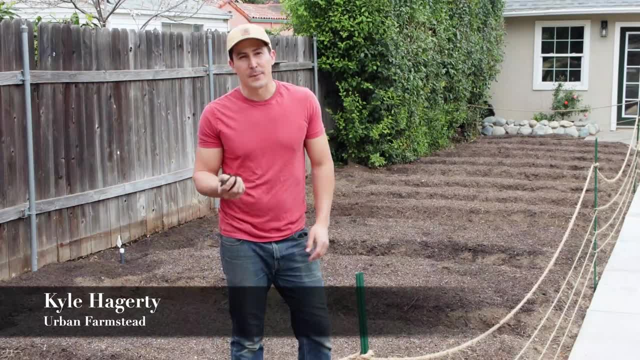 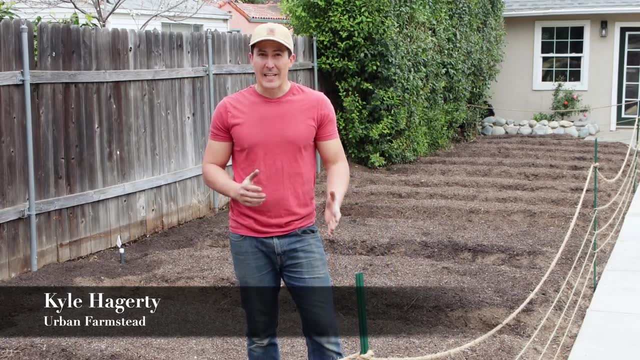 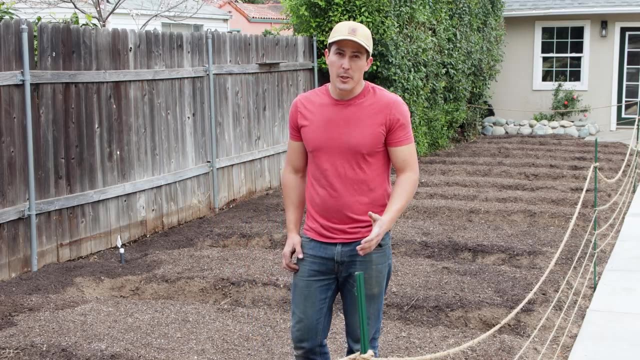 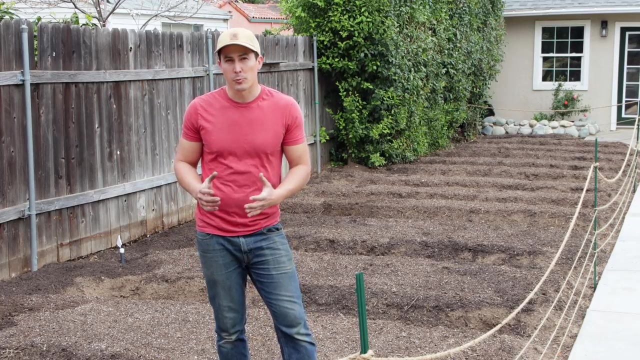 Soil is the most important investment you can make in your garden, And I'm not just talking about a financial investment. I'm talking about investing your time and energy to create and maintain healthy soil that will improve every season. I'm Kyle from Urban Farmstead, and in this video, I'm going to show you how to transform a yard full of weeds and poor soil into a fertile, vegetable plot capable of growing more produce per square foot, with less weeds, less disease, less irrigation and less fertilizer. 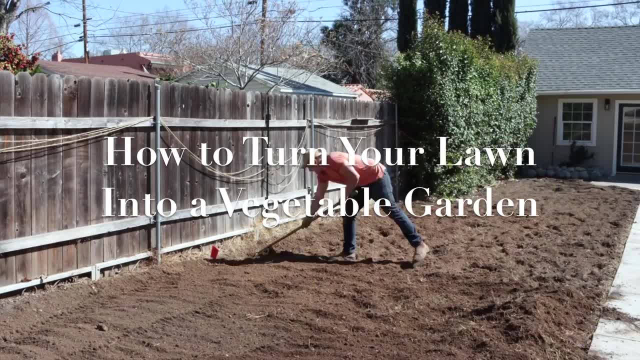 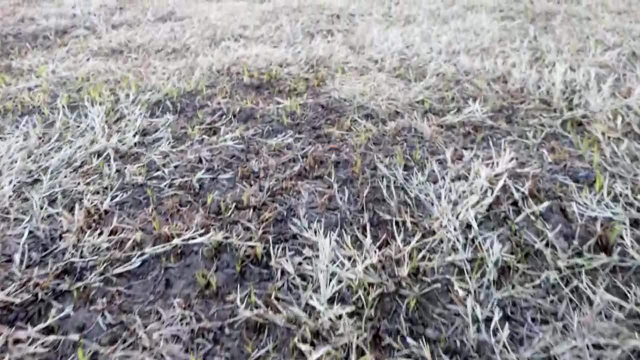 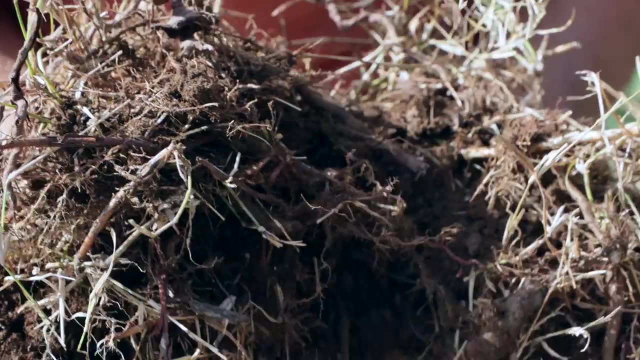 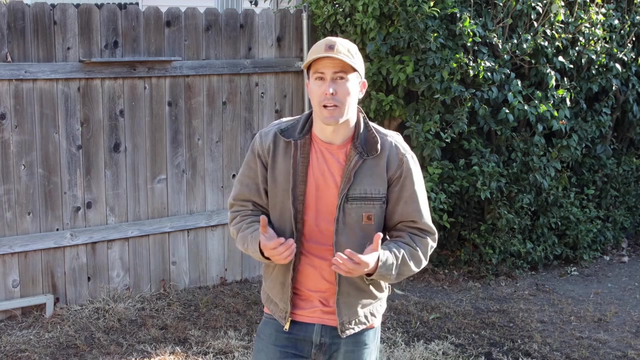 My very first step in preparing this soil for a new vegetable garden is going to be to remove as much of the existing weeds as possible, And really the roots of the weeds are what I'm trying to get rid of. Depending on the weeds that you have in your garden, your plan for the garden and your personal preference, your process might look completely different than mine. 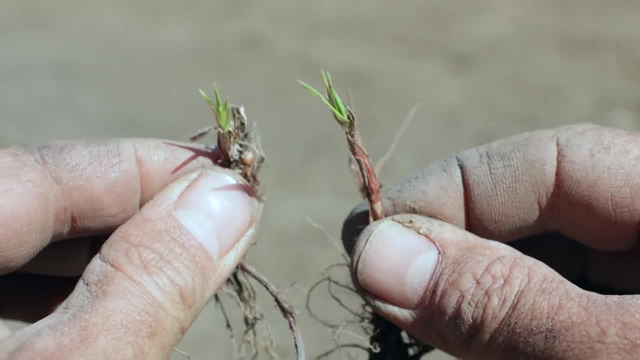 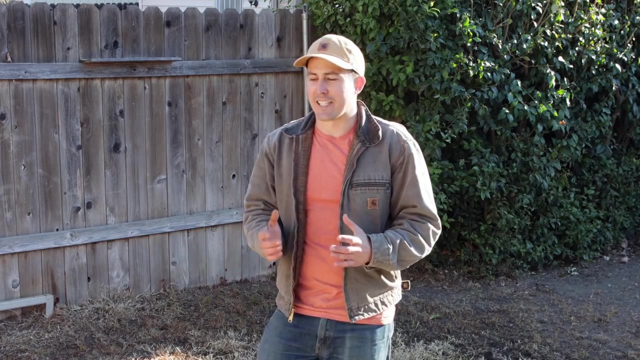 For me. I've got some really harsh weeds, like this Bermuda grass and yellow nutsedge, that honestly are almost impossible to get rid of, even with harsh chemicals. So my goal is not necessarily for them to be gone forever. That would be great, but I don't think that's going to happen. 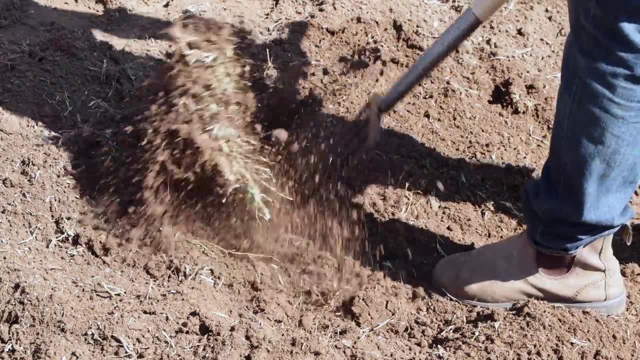 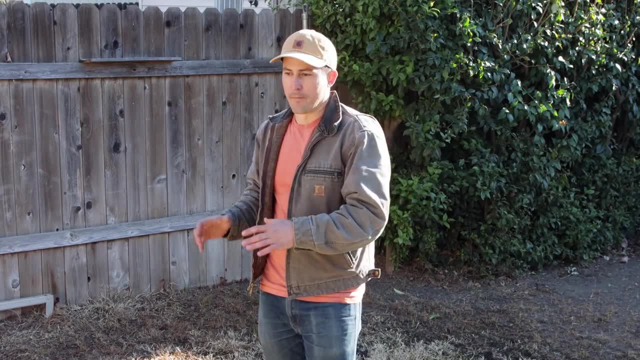 What I want to do is remove as much of their root mass as possible so that they don't come back as strong and so that my vegetables will still be able to thrive in this soil here. So what I've done so far over the last few months is sheet mulch over the entire area. 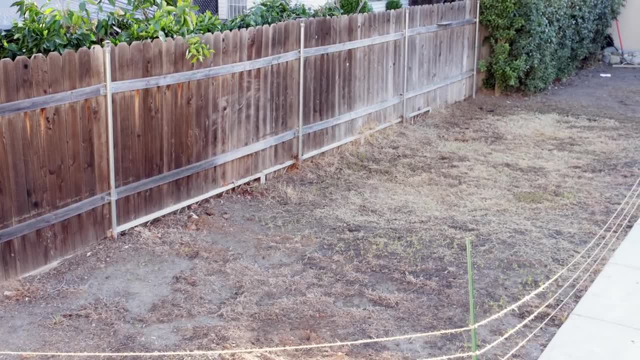 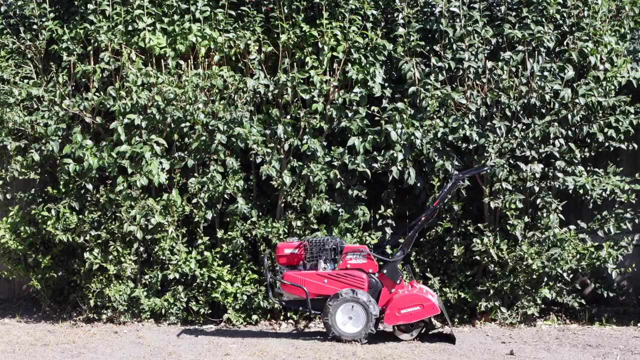 With a really thick layer of cardboard in order to deprive them of light, And that's not going to come anywhere close to killing them, but it takes some of the vigor out of them. Next, what I'll do is I'll come through, I'll rototill all of this and rake out as much of those roots as possible. 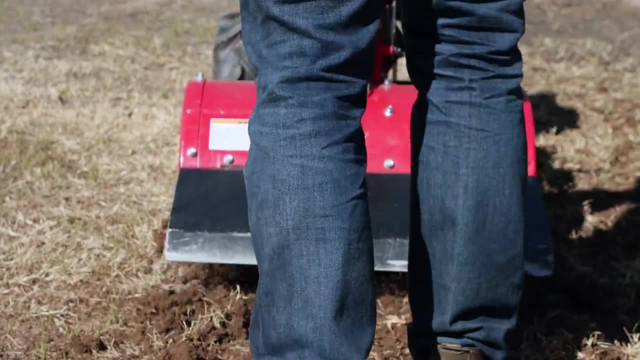 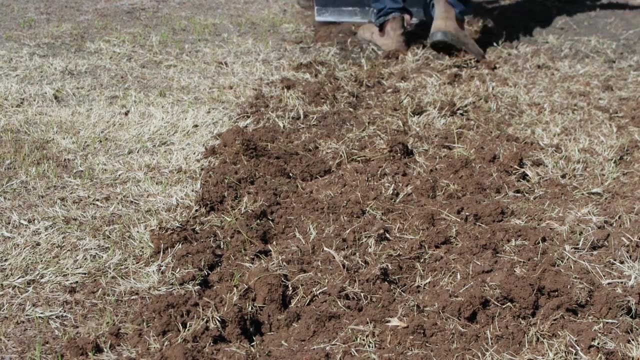 My goal here is not to do a full till, It's really just to loosen up the top few inches of this clay soil to make the weeds more easy to remove. The weeds that I have are very invasive, but the roots are actually pretty shallow. 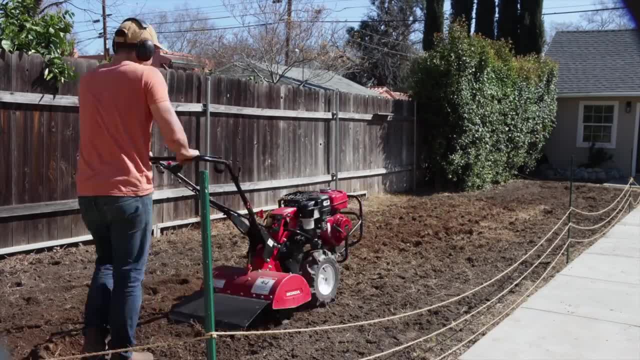 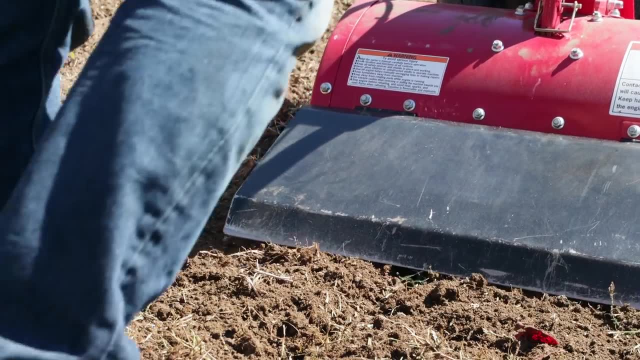 That's a characteristic of these weeds and the heavy clay soil that they're growing in. If these were growing in sand, they'd have much deeper roots. If your garden has deeply rooted rhizomatic weeds, like fine weed, they should be removed prior to tilling. 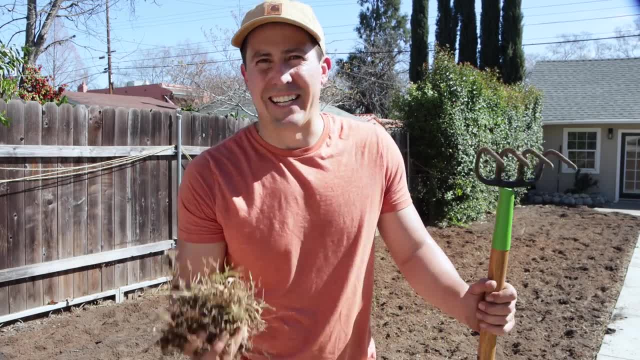 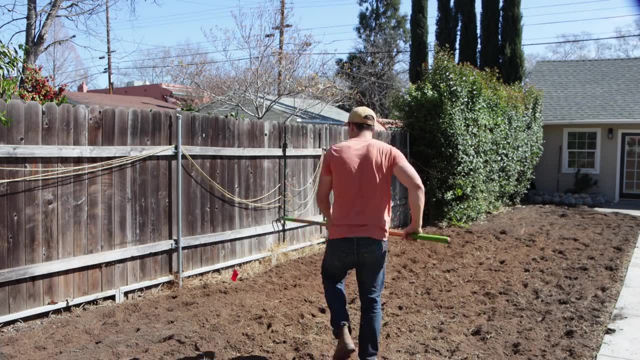 Alright, I've tilled all of this soil twice. I've loosened it up a lot. Now I'm just going to rake through and remove as much of these grass clumps and weed roots as possible. Some people choose to completely remove the top few inches of soil containing the roots and seeds of the weeds. 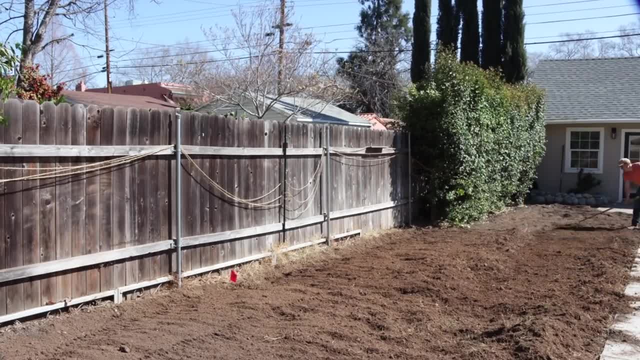 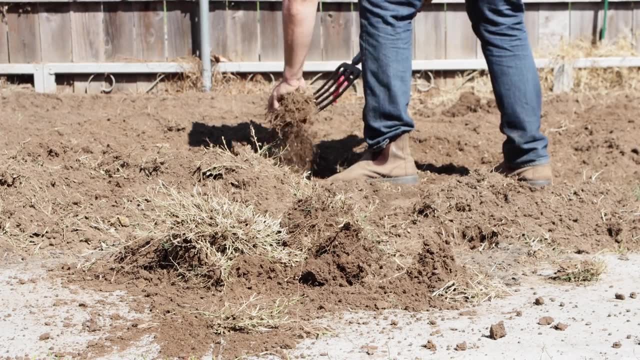 That process is just as effective, But it requires hauling off a lot of material, And those top few inches are the most valuable layer of your topsoil. Raking out only the weeds is more labor-intensive, But for me it's worth that extra effort to save this nutrient-rich native topsoil. 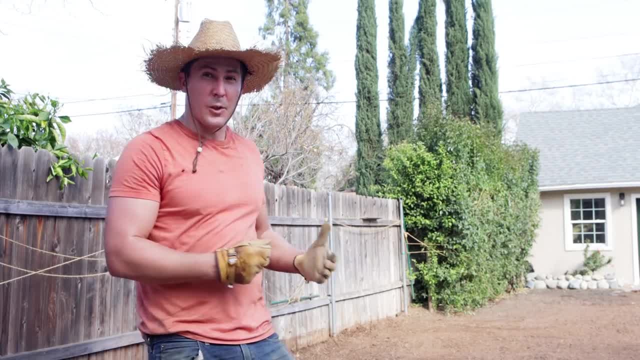 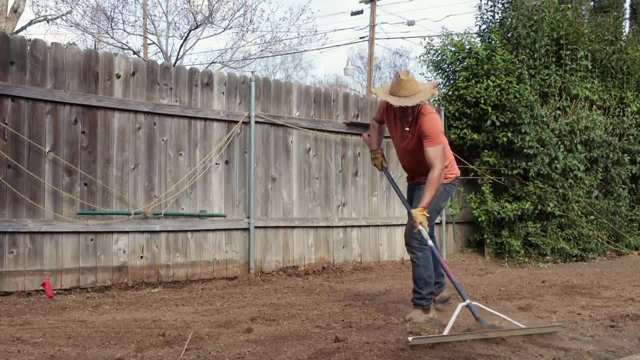 Alright, step one is complete. I've removed a lot of those grass roots and those weeds. There's still going to be plenty of them left in the soil. I've definitely tilled some of those weed seeds back into the soil, So there's going to be stuff coming up. 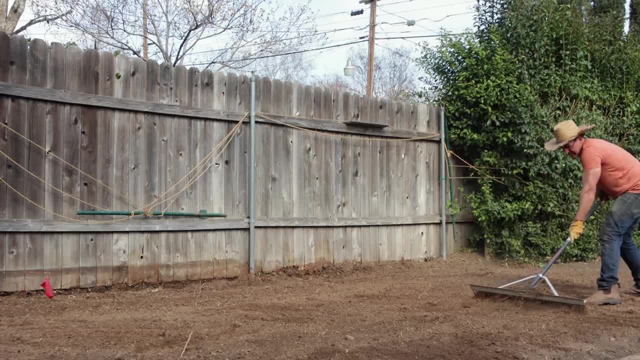 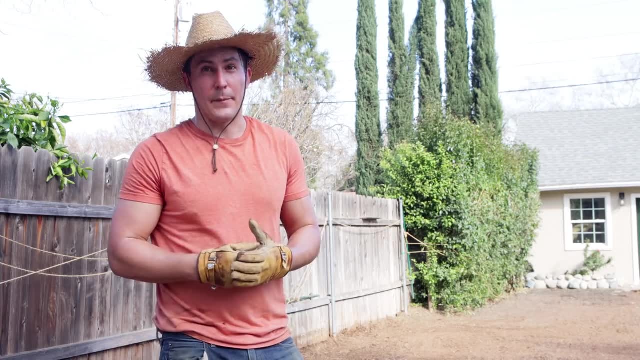 But from my experience at our last garden, I did the exact same thing And it worked really well. It really brought the weed amount down And once I mulch over the top we're not going to have very much coming up at all. 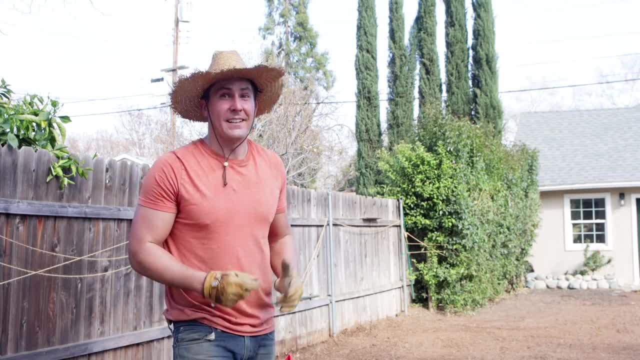 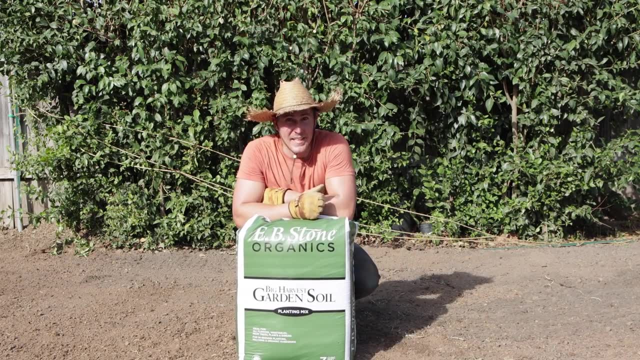 You might choose to do something different with your garden. This is what I did with mine. It's going to work well. Next step is to bring in some compost. Anytime you're amending soil for a vegetable garden, the very best thing you can do. 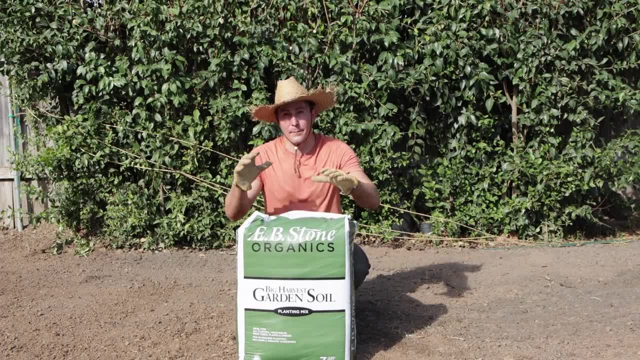 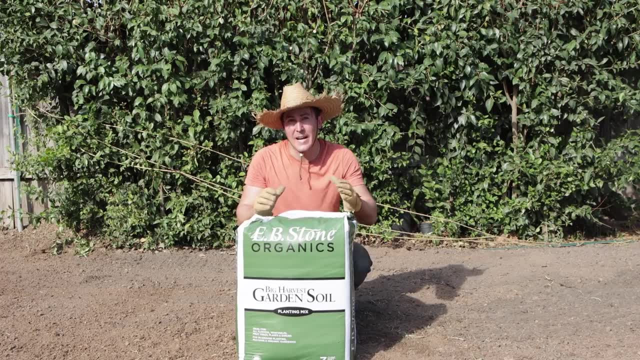 is add organic matter, And that can be bulk compost, It can be bag compost, It can be compost you make in your own backyard. It can even just be wood chips or leaves or pine needles. Whatever you add is going to be great. 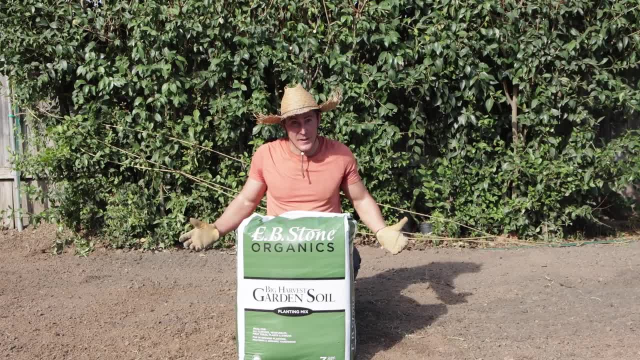 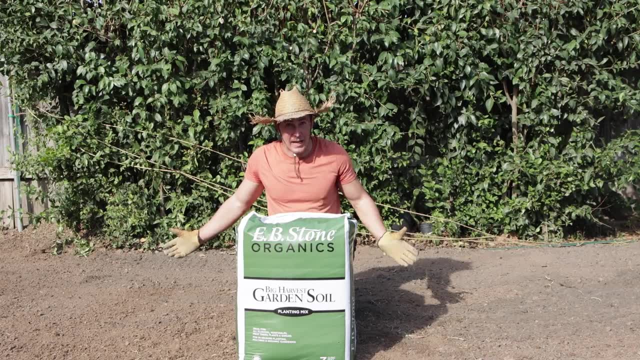 But for me, when I'm doing a very important project like our brand new vegetable garden, I want to add the very best compost and I want it to have even more nutrients in it. This is just regular topsoil that I'm adding to. 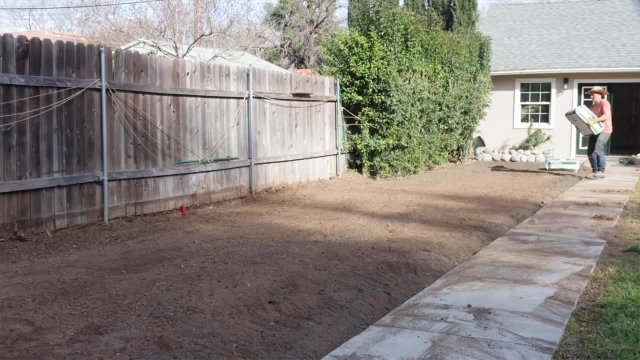 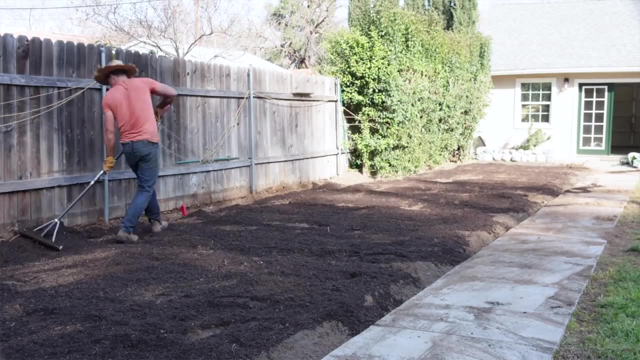 So this bag has not only regular aged redwood and fir bark, it also has dehydrated chicken manure, earthworm castings, bat, guano, kelp meal, alfalfa meal, All kinds of stuff that's not only going to add that organic matter to my soil. 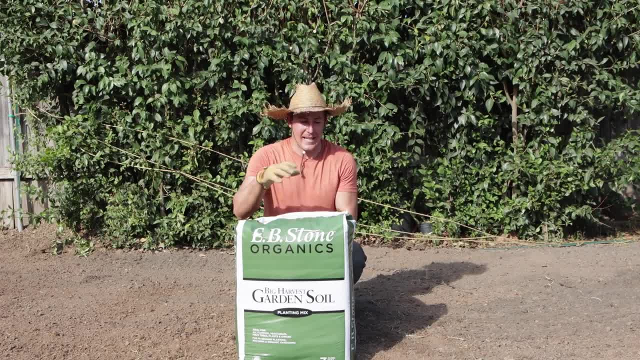 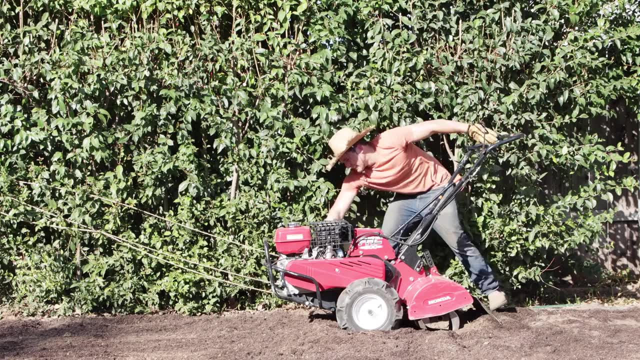 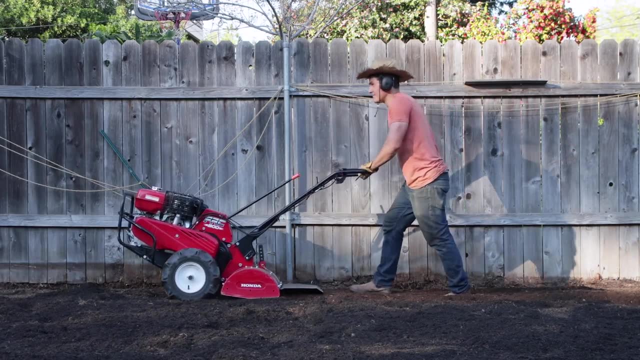 but it's also going to add a lot of nutrients to my soil And it's going to help it build some really good microbes and have a really, really healthy garden this year. So let's till this in. I am a huge proponent of no-till farming practices and no-dig gardening. 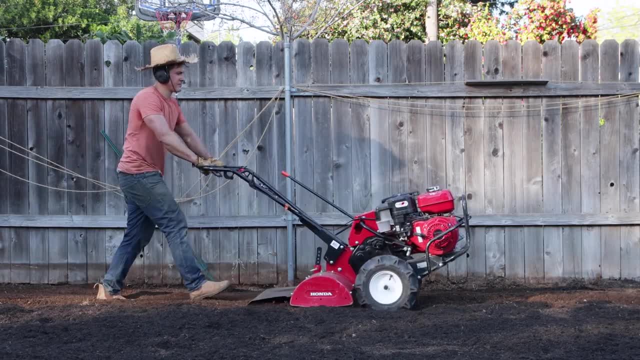 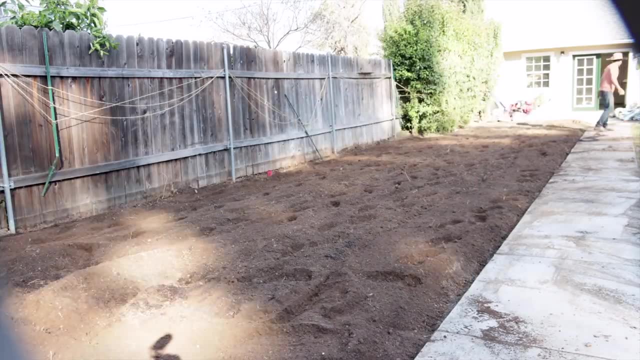 And we'll absolutely be using those methods here, as I do on our other farmstead. But when starting a new garden in either heavy clay soil or very sandy soil, it's often recommended to establish your soil structure that first season by tilling in compost. 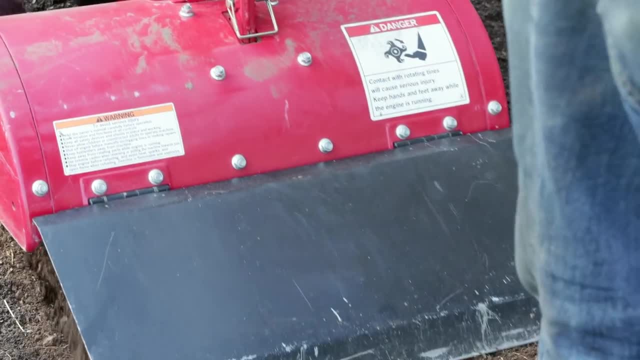 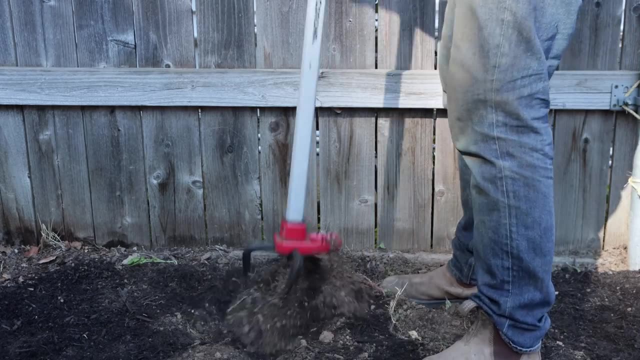 And then never tilling after that. From now on, any soil amendments I add to this plot will be applied directly to the soil And I'll allow the soil microbes and beneficial bacteria to establish and maintain the soil structure. This soil ripper from Corona Tools is perfect for loosening soil in the areas I can't get to. 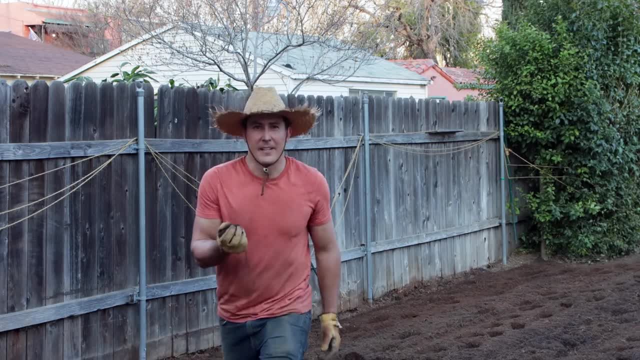 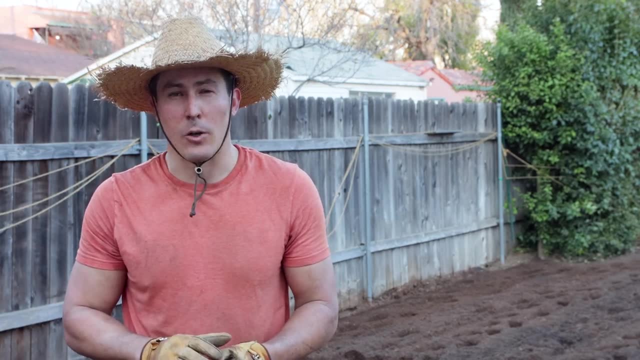 with the tiller. Alright, all that compost is tilled in and the soil is looking great. The next thing I need to do is shape all of these beds, And then I'll add an extra layer of soil amendments on the top of each bed and mix that in. 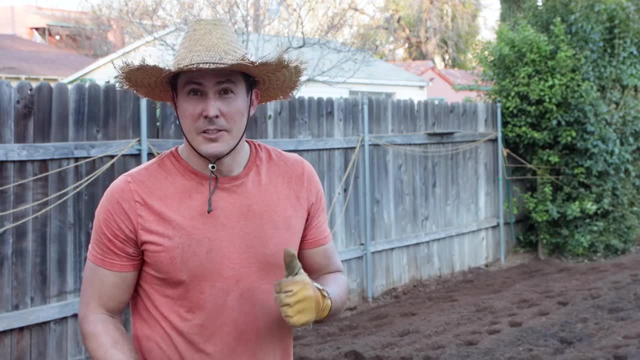 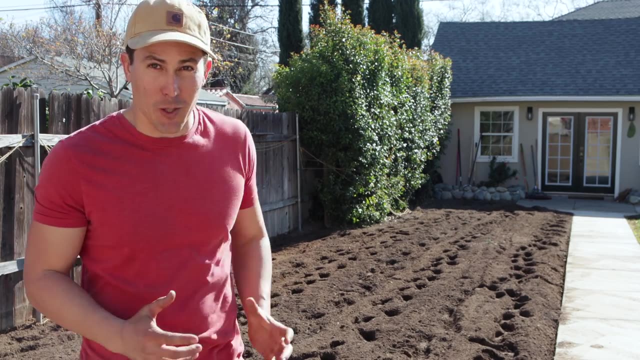 But it's getting a little late. I've got to get that rototiller back to the rental place, So let's pick up here tomorrow. Alright, it's day two, and I am really excited because today will be the first time that this plot of soil will finally start to actually look like a garden. 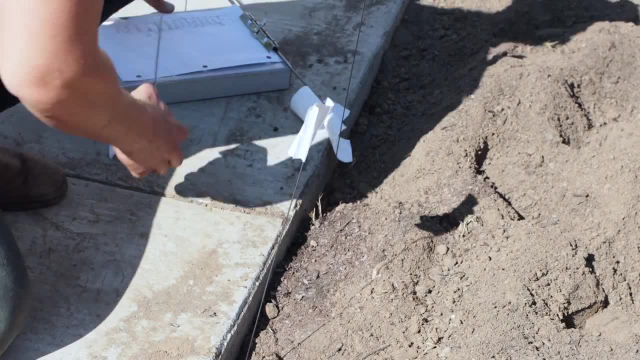 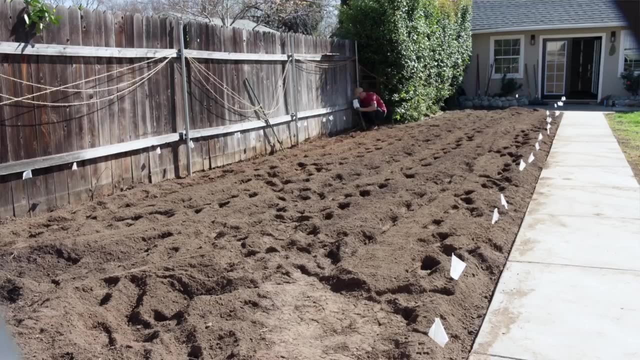 I've already measured this entire spot And drawn up a sketch to scale that shows the size and spacing of each bed For permanent gardens, especially with hardscaping like raised beds built out of wood or cement. I like to make my pathways wide enough that I can push a wheelbarrow down them. 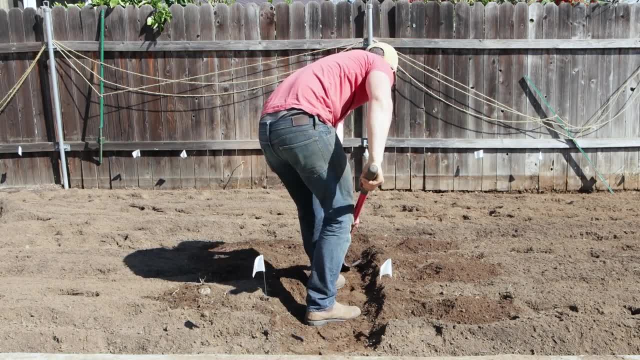 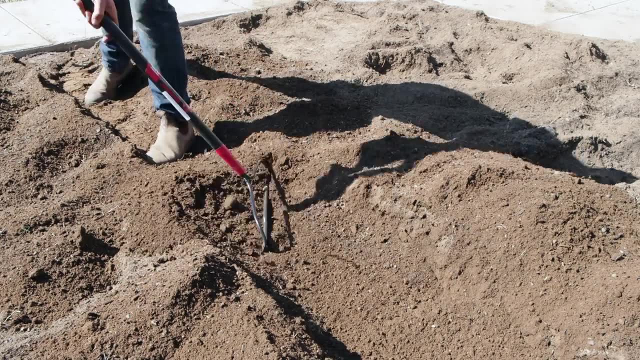 But this is sort of a temporary garden, so I'm making my pathways a little bit more narrow. They're only going to be 18 inches wide, which will allow me access to walk down them, but not necessarily get a wheelbarrow all the way down them once the crops have filled in. 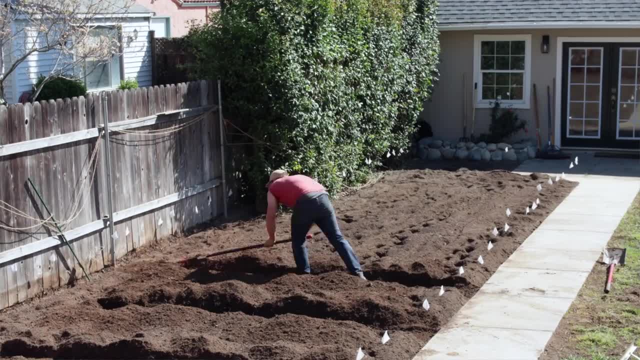 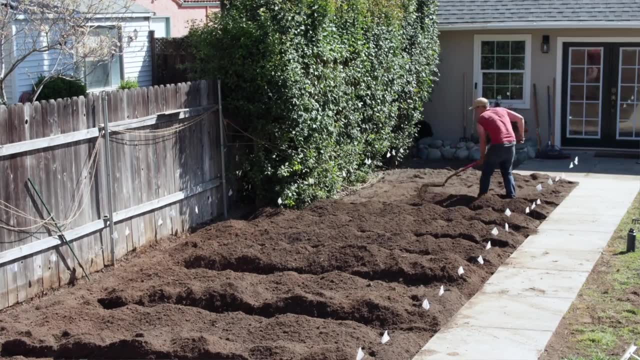 The beds, though, will have low-growing freestanding crops Like peppers and summer squash, will be four feet wide, which is wide enough to grow a lot of vegetables in them, but not so wide that I can't reach into the center without stepping on and compacting the soil. 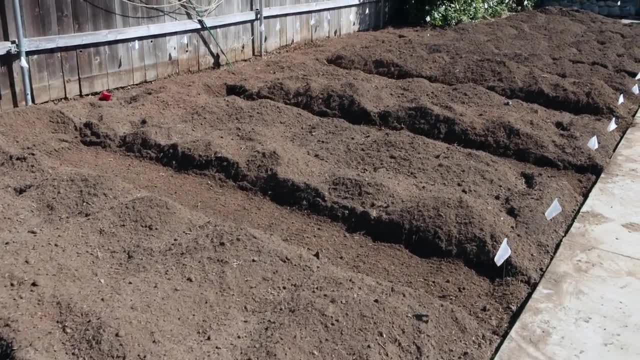 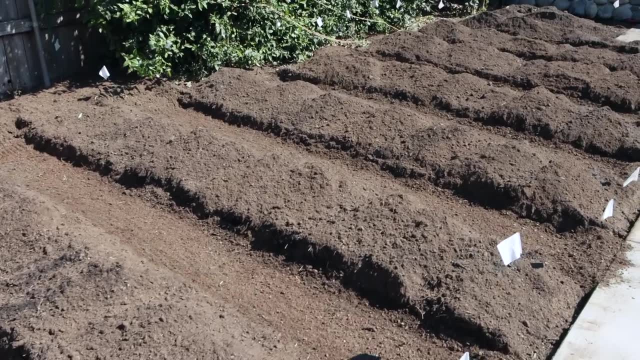 Taller crops that I'll grow on trellises, like tomatoes, tomatillos, beans and cucumbers. those beds will be two feet wide so that I can run a trellis down the center and still access that trellis from both sides. 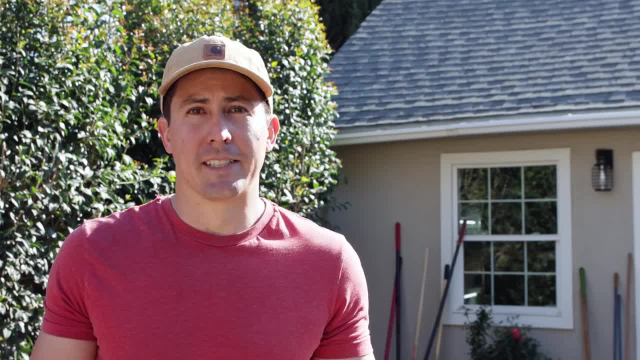 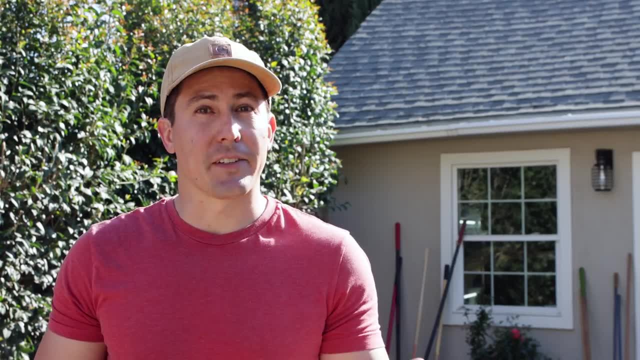 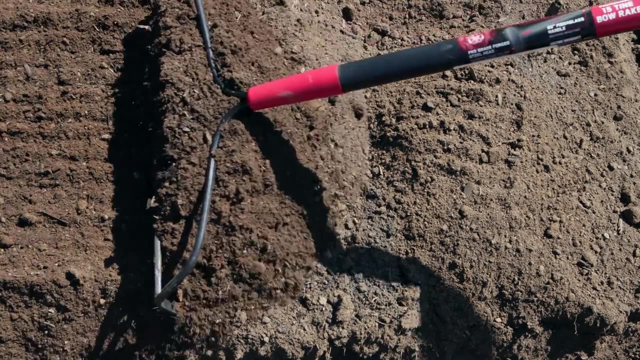 Creating a bunch of small beds rather than a few large beds allows me to grow each crop in their own specific area, Which has a lot of advantages, including amending the soil specifically to that crop and crop rotation. Orienting my beds north to south will provide them the best opportunity for maximum sun exposure. 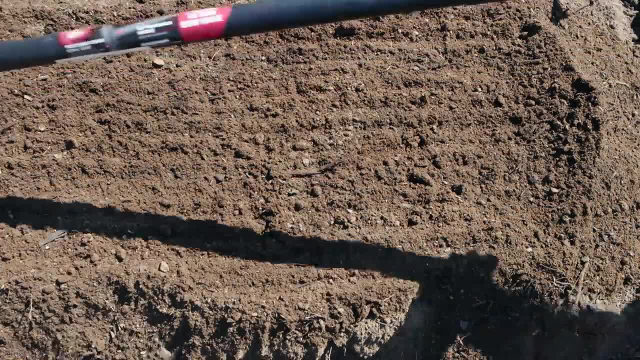 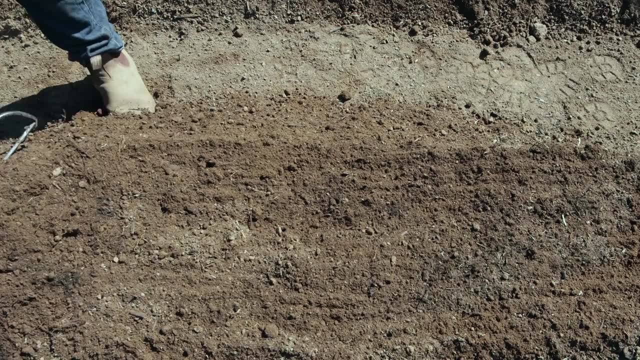 I could orient the beds east to west if that was my only option, but it's likely to create a situation where I've got inconsistent sunlight, with some areas of the garden being scorched by the sun and other areas being shaded out, And it really reduces my options for what I can plant where. 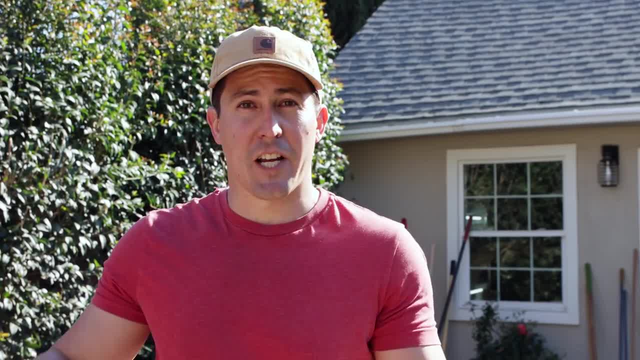 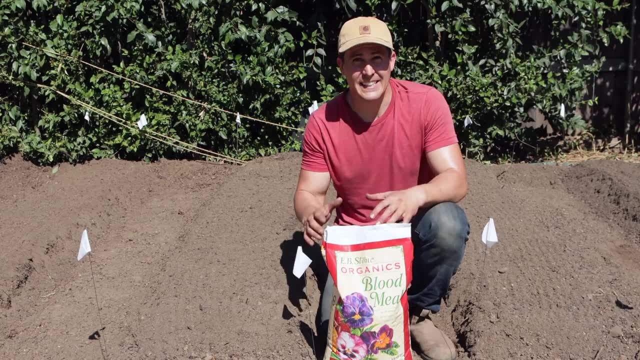 because if I planted taller crops in the southern beds, it would shade out the plants of the northern beds. Alright, so I've mixed in a bunch of compost, I've shaped the beds. now it's time to add the exact soil amendments that I need in order to get my soil ready to grow my crops. 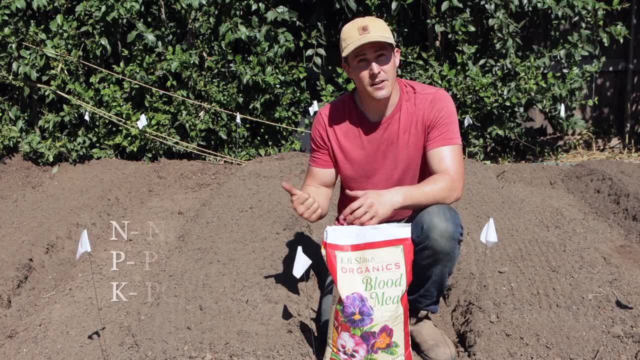 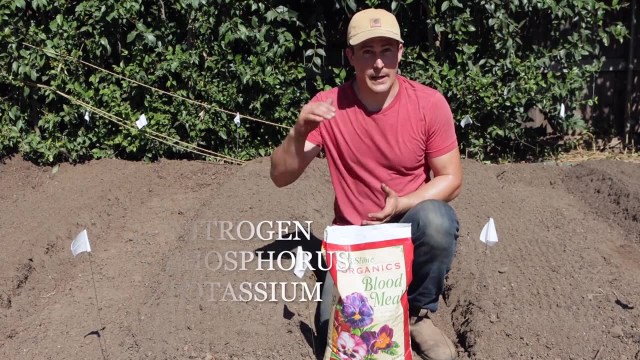 Now there's three main nutrients known as macronutrients, and they're nitrogen, phosphorus and potassium, And in most cases, a lot of those are already existing in your soil. but they're all at different levels, sometimes too high, sometimes too low. 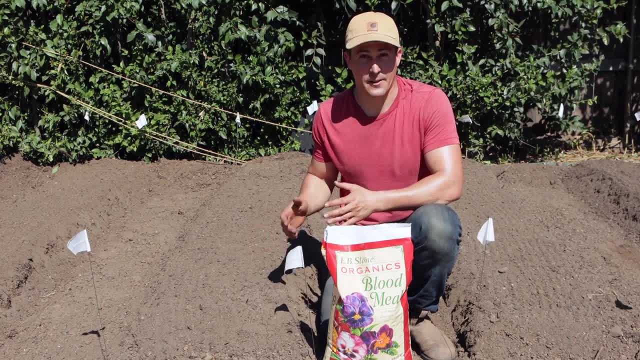 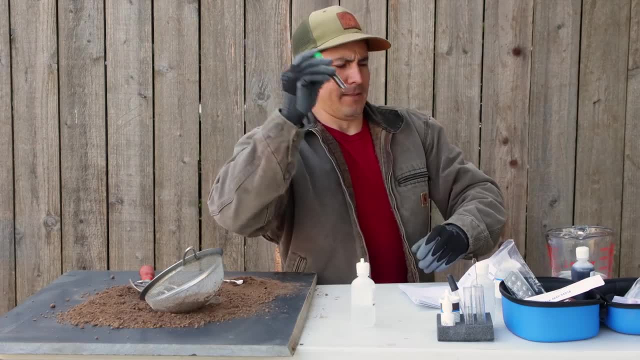 And the best way to determine what levels they're at is to have your soil tested. You can set it off to a lab for an analysis or use a home test kit Now. I recently did a video on exactly how I tested my soil. 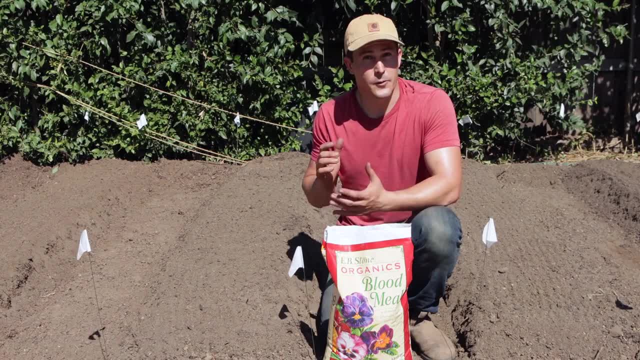 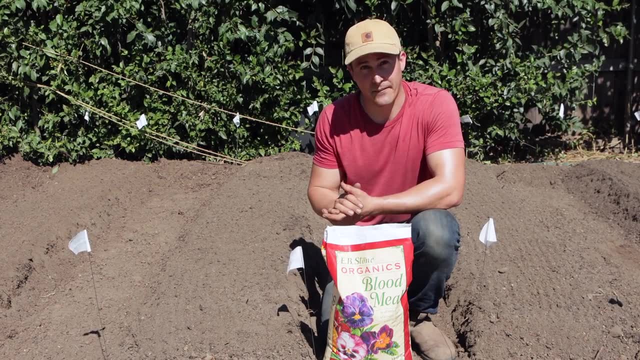 I trialed a few different kits and I sent one off to a lab and compared everything. So if you want to see how I tested my soil and get an idea of what some good kit options might be for home testing, I'll add a link to that video here. 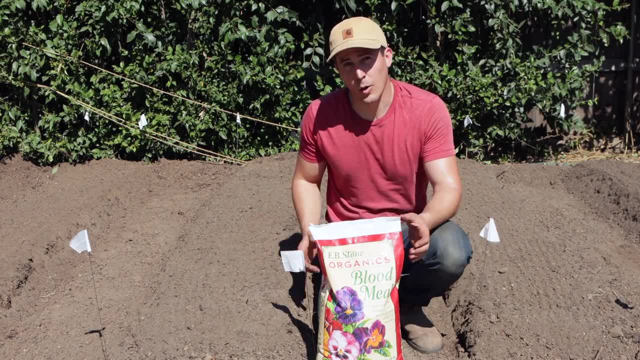 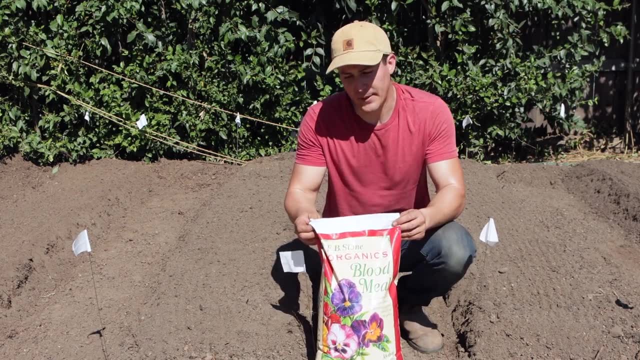 My soil test determined that the nitrogen levels in this soil is on the lower end, So I'm going to be adding some organic nitrogen fertilizer to amend this soil. This is an organic blood meal from EB Stone and it's basically a slow-release nitrogen. 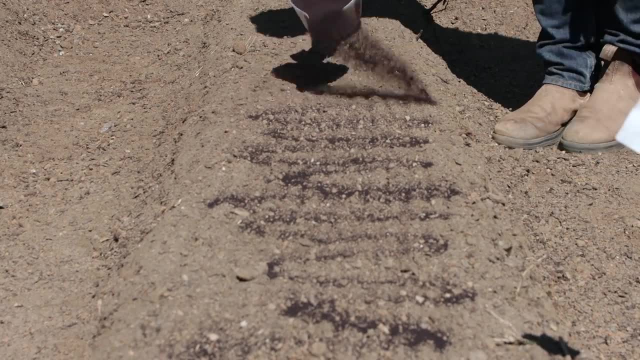 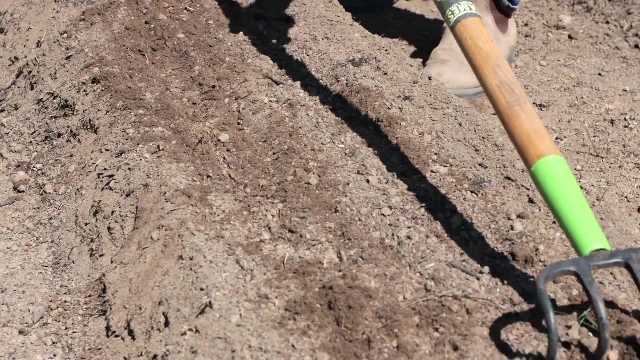 It's a 13-0-0.. That first number is the nitrogen. so lots of nitrogen. I'm just going to add this on top of the soil, mix it in a little bit and it's going to be a great slow-release nitrogen that will last the entire season. 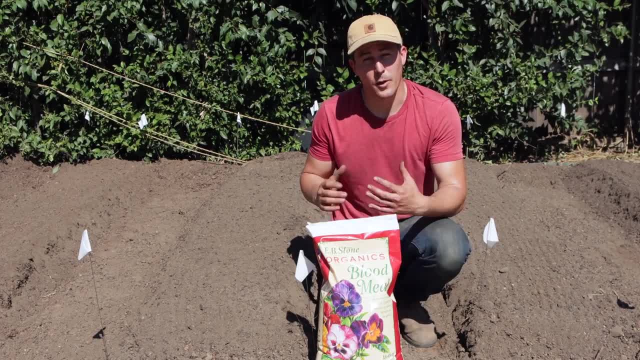 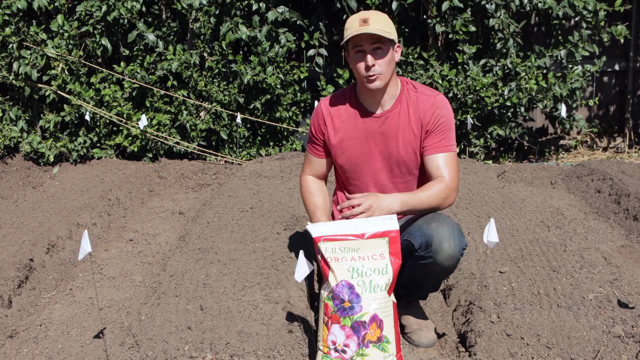 Starting your garden with organic soil amendments and maintaining it with only organic fertilizers is the best way to build and sustain live, healthy soil, and your plants will reflect that All right. one last soil amendment. This stuff is like the icing on the cake. 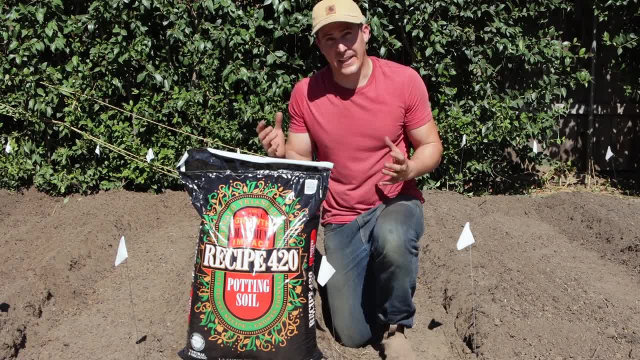 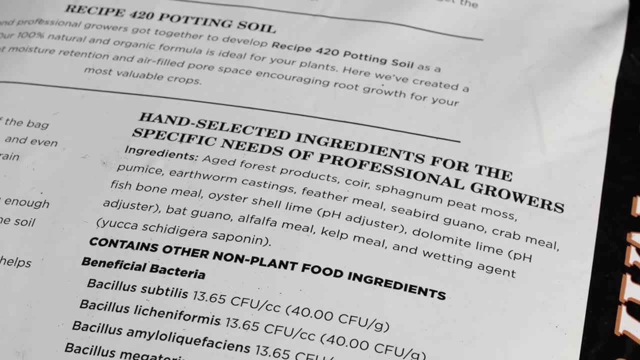 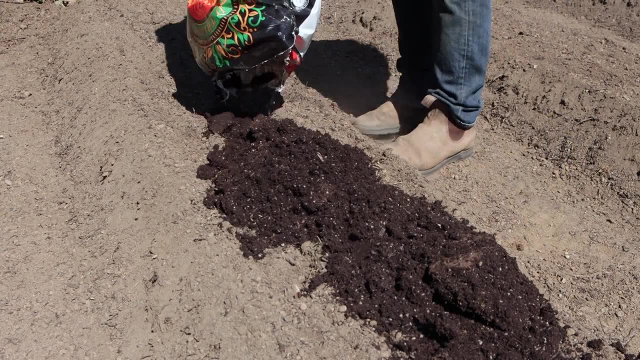 This is called Recipe 420, and it's like this elevated organic potting mix. Not only does it have a broad range of really nutrient-rich organic matter, but it also has beneficial bacteria and mycorrhizal fungi. This stuff is going to just be added on top of these beds, just like that blood meal was. 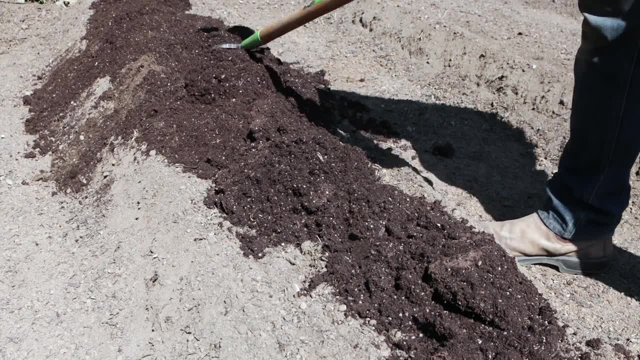 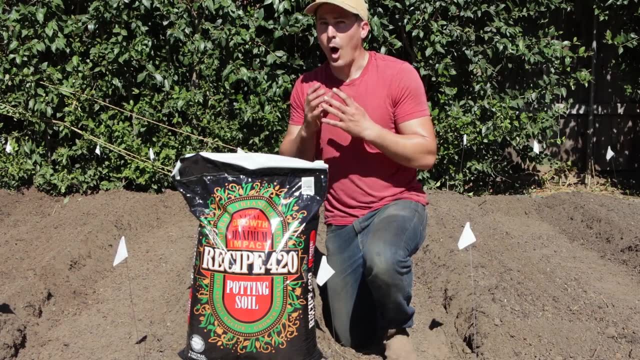 I'll barely scratch it in- and it's going to create an environment for the roots of the new plants to thrive and it's going to continue to break down and feed the soil and the vegetables growing in it all season long. If you can find this at your local nursery, I highly recommend it for top dressing your beds. 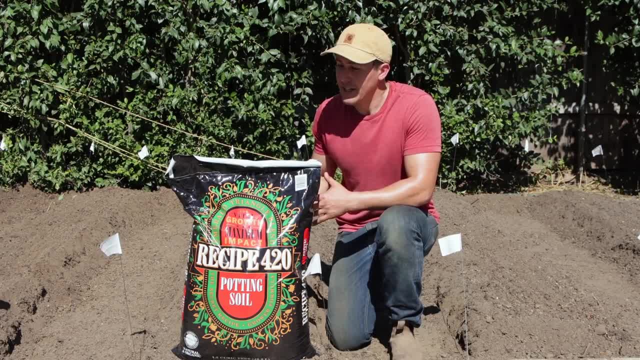 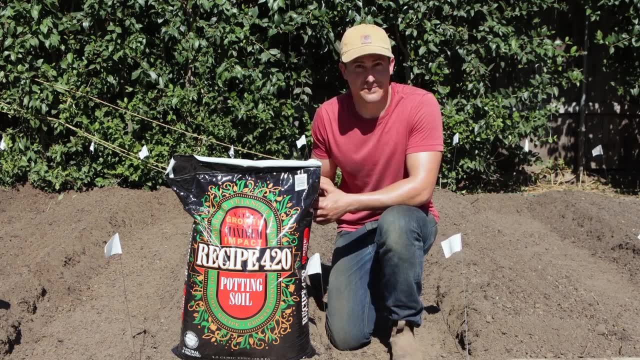 not only the first season, but each season after that. before you plant Now, if you can't find this product in your area, I recommend just using the most high-quality compost or potting mix that you can find, In addition to building your soil structure and balancing the nutrients. 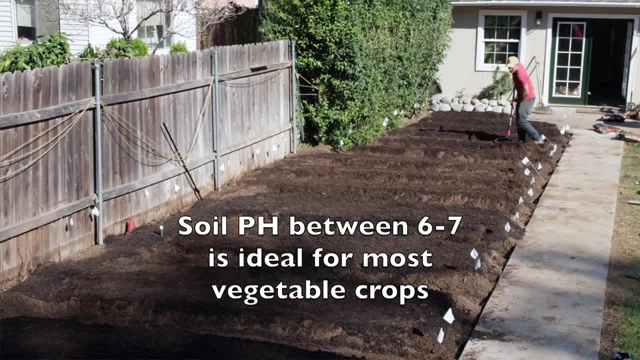 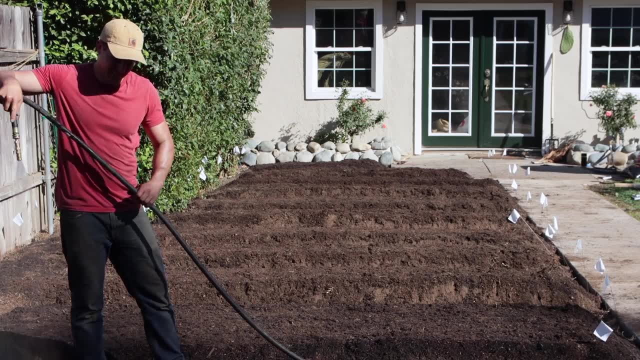 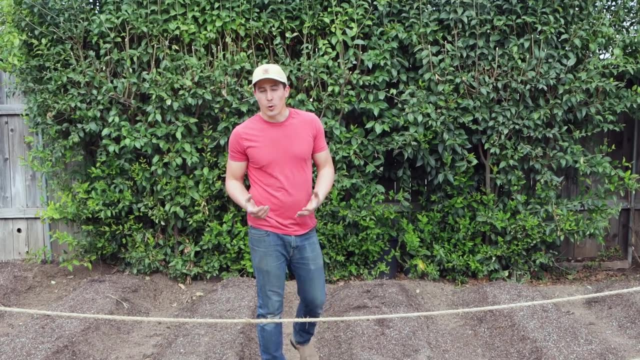 now's the best time to check your soil pH and adjust it if necessary. All right, the only thing left to do now is water it all in Now. I'm going to allow the soil to settle for a few weeks and during that time, I want to encourage any of the weed seeds or rhizomes. 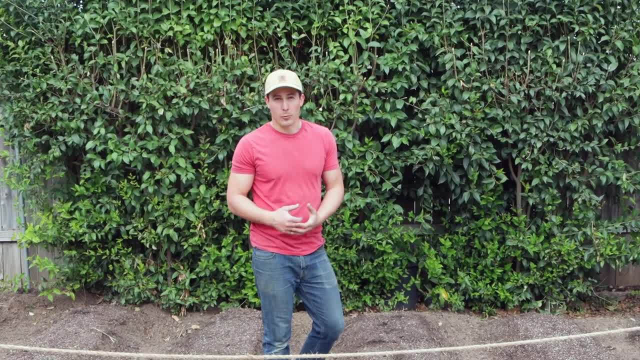 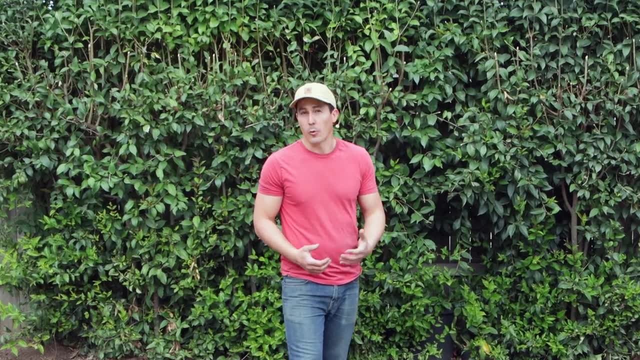 from those weeds that are left in the soil to germinate And with rain in the forecast and a little bit of sunshine, it should create the ideal spring conditions to germinate those weeds so that I can pull them before planting. All right, it's been a few weeks now since I built these beds. 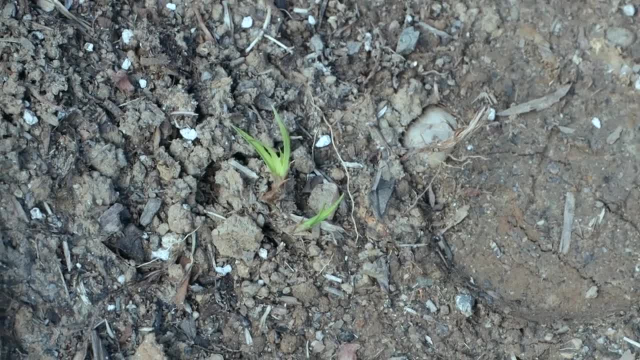 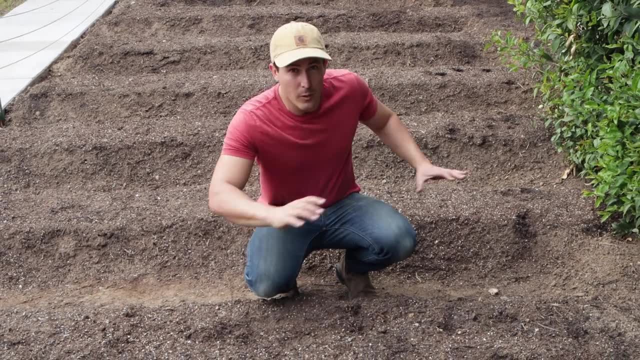 and we got that rain and the sunshine that were forecasted, but we didn't get very much. There were a few here and there that I plucked out, but it was encouraging to see that this area that was before full of weeds now has pretty much none. 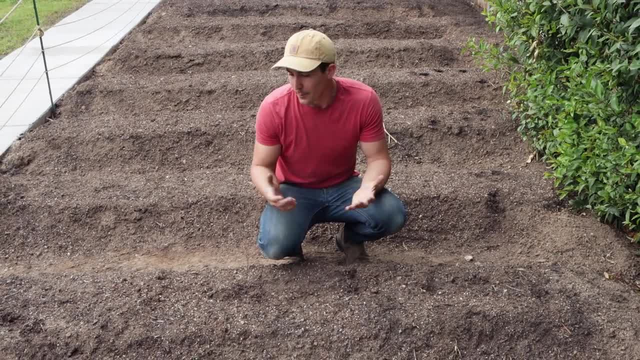 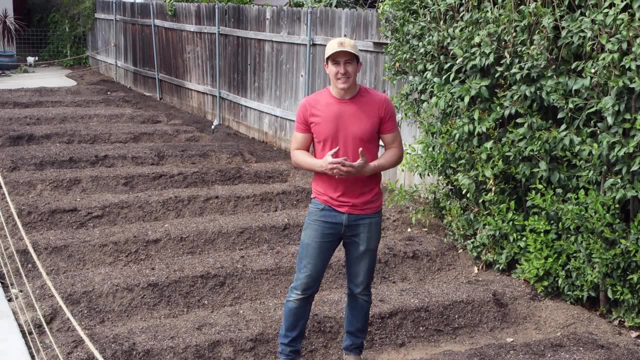 And I know there's going to be some that will continue to come up after planting, but at this point I can see that this plot is ready to plant. It takes time to build healthy soil, because great soil is not just the right blend of organic matter and minerals. 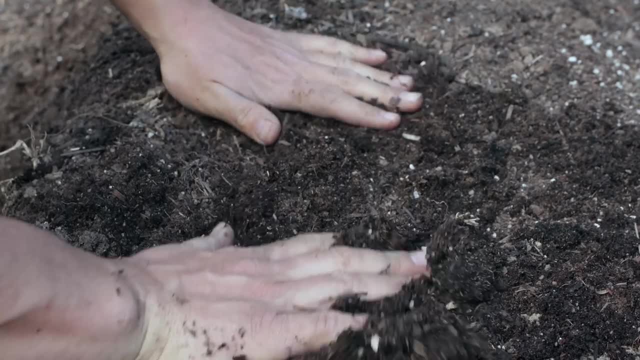 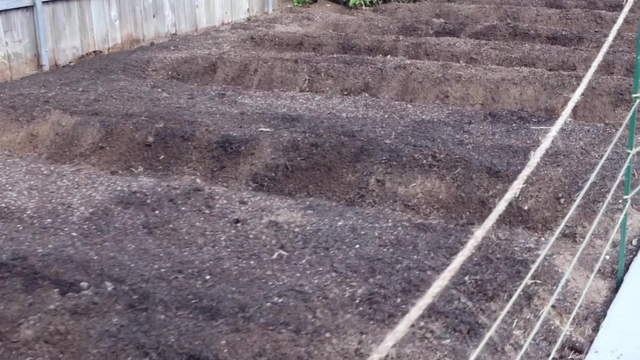 Healthy soil is alive, just like the plants that it's feeding, so it relies on the microbes and other microscopic organisms within the soil that form a symbiotic relationship with your plants. So continue to manage your soil by feeding it regularly with organic fertilizers. 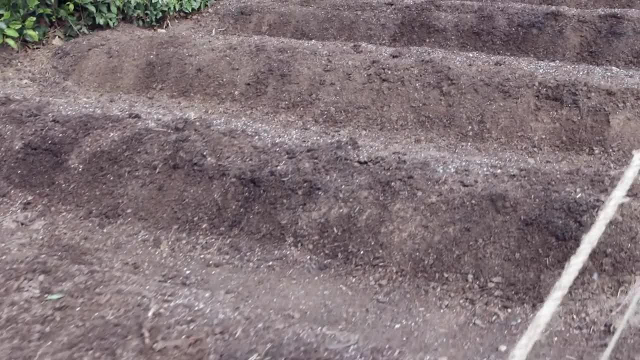 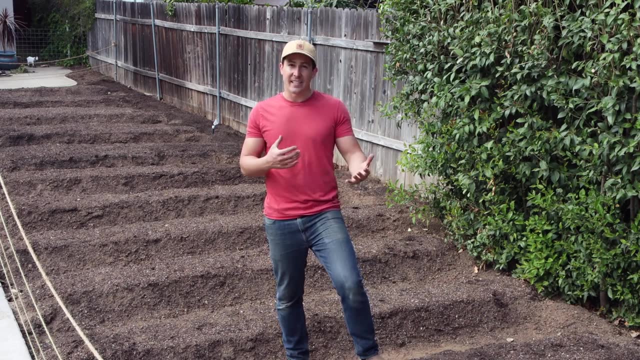 maintaining the soil structure by adding compost each season, never tilling after the initial till and reducing soil compaction by not stepping on the beds and also planting cover crops during the rainy season. Those basic soil management practices will allow you to grow more produce.